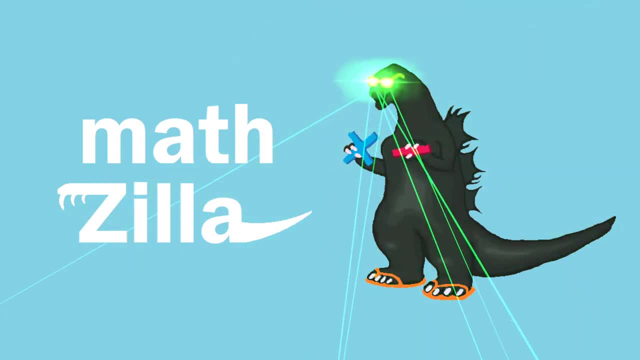 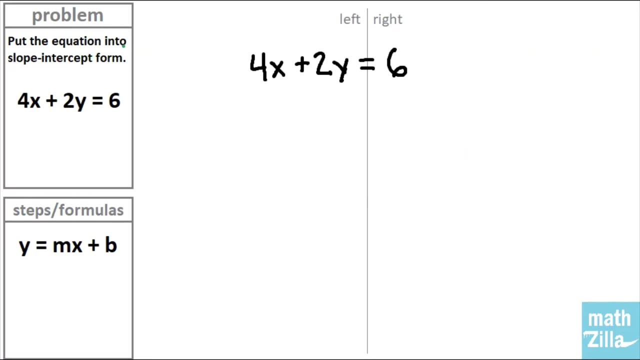 Hey everyone, how's it going? Today we're going to look at a common slope-intercept problem. Put the equation into slope-intercept form: 4x plus 2y equals 6.. In order to do this, we need to know that slope-intercept form is: y equals mx plus b. As you can see in slope-intercept. 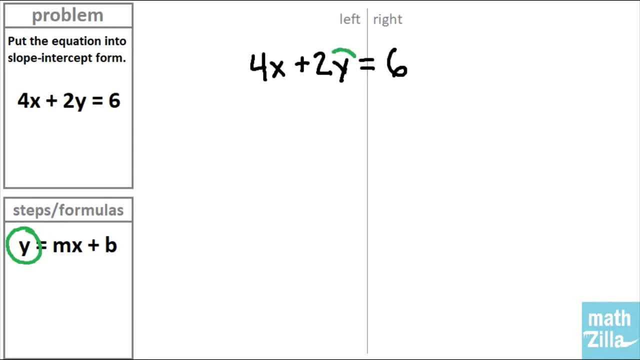 form, the y variable is all by itself. So in our problem we need to copy that and get the y variable all by itself. on the left-hand side, That means we need to cancel out the 4x and the 2.. Let's start with canceling out the 4x. Well, this is plus 4x. 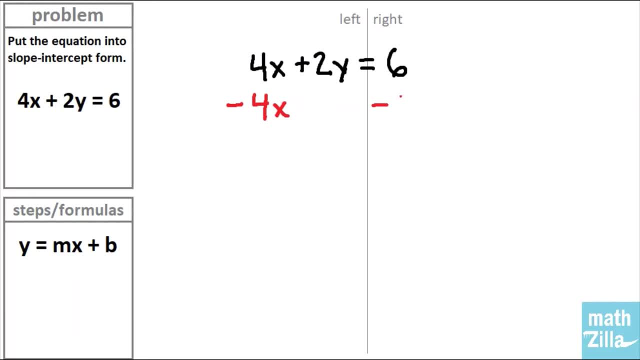 so we do the opposite and we subtract 4x from both sides. On the left-hand side of the equation, 4x minus 4x cancels out and we're just left with 2y. On the right-hand side of the equation, we now have negative 4x plus 6.. Continuing to get the 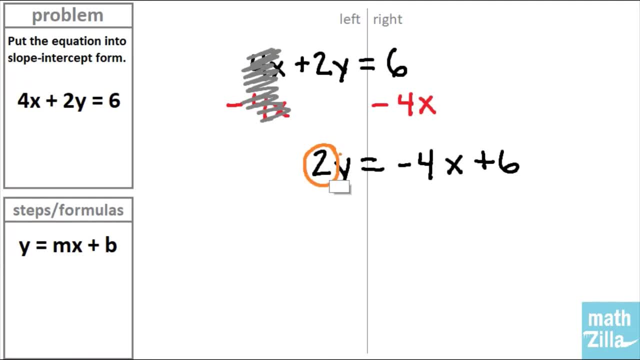 variable y all by itself. we now need to cancel out the 2 on the left-hand side. This is 2 multiplied by y. so in order to cancel out, we do the opposite: divide by 2 on both sides of the equation. 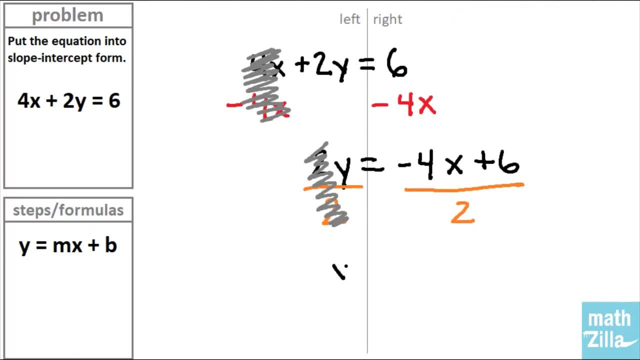 On the left-hand side, the 2s cancel out and you're just left with y. On the right-hand side, we have negative 4x divided by 2, which is negative 2x, and we have 6 divided by 2.. 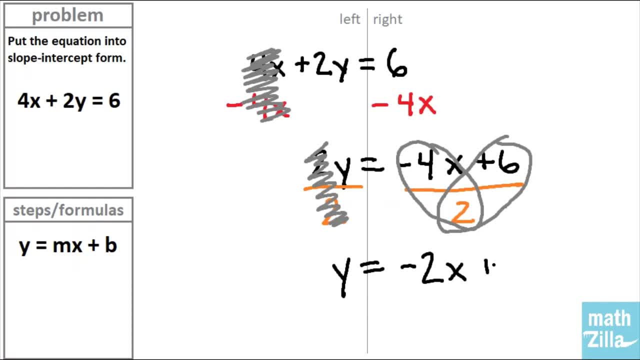 6 divided by 2 is plus 3.. Our answer is: y equals negative 2x plus 3.. Let's check our work. Mathzilla always checks his work. If we compare this to our slope-intercept formula, you can see that our answer and the formula are now matching.